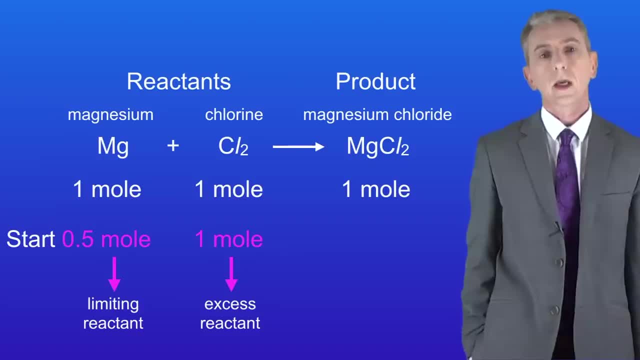 excess reactant, and that's the chlorine. So let's see what would happen in this reaction. As the reaction proceeds, the magnesium would all get used up. We would use up 0.5 moles of the chlorine and we'd make 0.5 moles of. 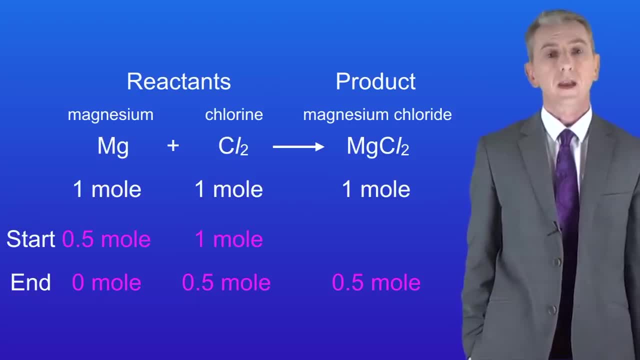 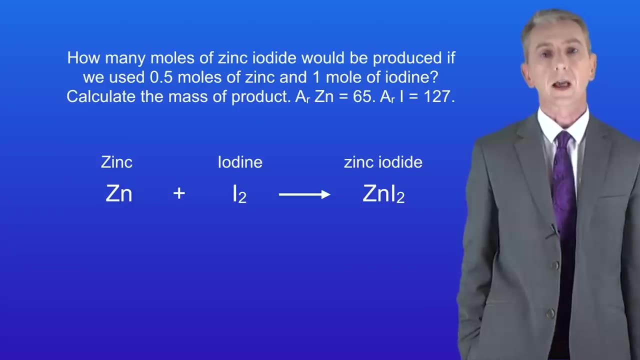 magnesium chloride. Now in the exam, you could be asked to predict the outcome of a reaction, taking into account which reactant is in excess and which is limiting. Let's look at a typical question: How many moles of zinc iodide would be produced if we used 0.5 moles of zinc and? 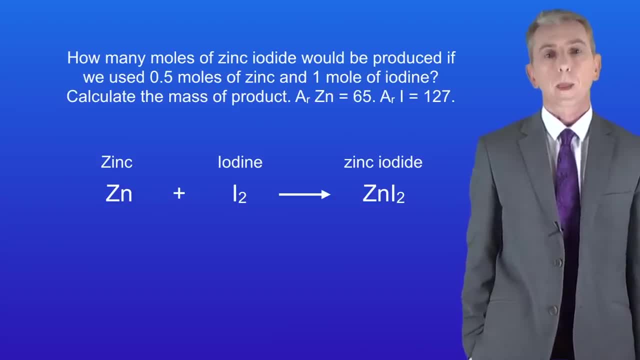 1 mole of iodine, Calculate the mass of product. Looking at the chemical equation, we can see that 1 mole of zinc reacts with 1 mole of iodine to make 1 mole of zinc iodide. We'd be given 0.5 moles of zinc, which makes that the limiting reactant. That means that we 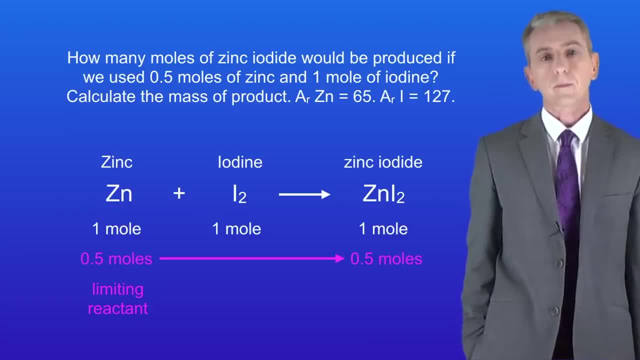 must make 0.5 moles of zinc iodide In this reaction. the amount of iodine has no effect on the amount of product because the iodine is in excess. There'll be some iodine left over at the end of the reaction. The question also asks us to calculate the mass of product. 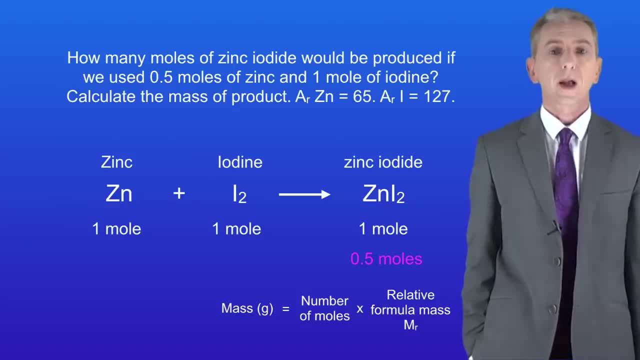 To do this we use the equation: mass equals number of moles multiplied by relative formula. mass Zinc iodide is 319.. Multiplying 0.5 by 319 gives us a final mass of 159.5 grams. Here's a question for you to try: How many moles of sodium chloride will be produced if we 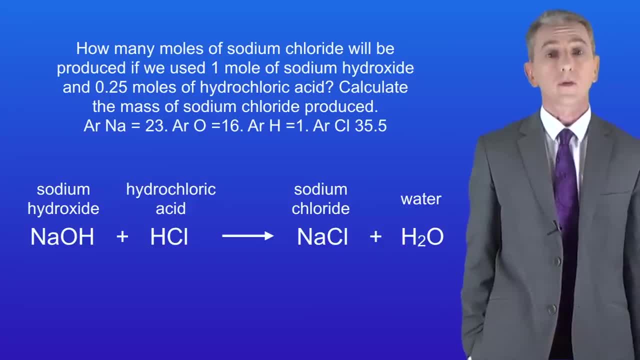 used 1 mole of sodium hydroxide and 0.25 moles of hydrochloric acid, Calculate the mass of sodium chloride produced. Pause the video now and try this yourself. Looking at the equation, we can see that 1 mole of sodium hydroxide reacts with 1 mole of hydrochloric. 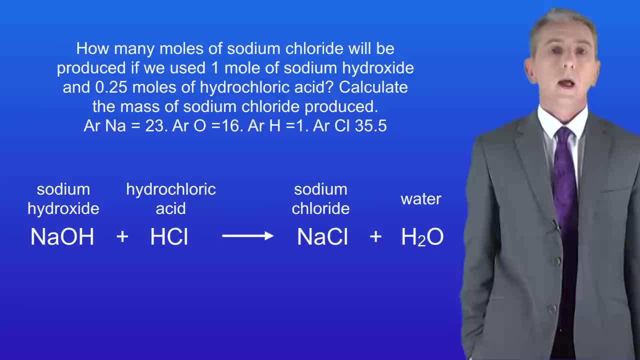 acid to make 1 mole of sodium chloride. Because we're only using 0.25 moles of hydrochloric acid, this makes the hydrochloric acid the limiting reactant. This means that we can make 0.25 moles of the sodium chloride. To work out the mass, we multiply the number of